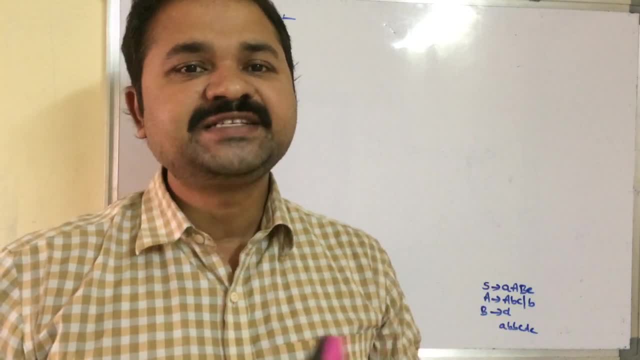 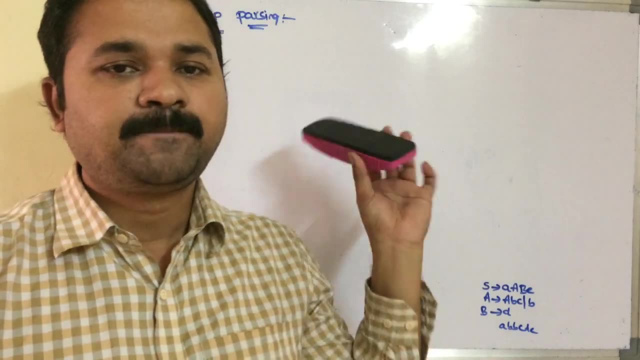 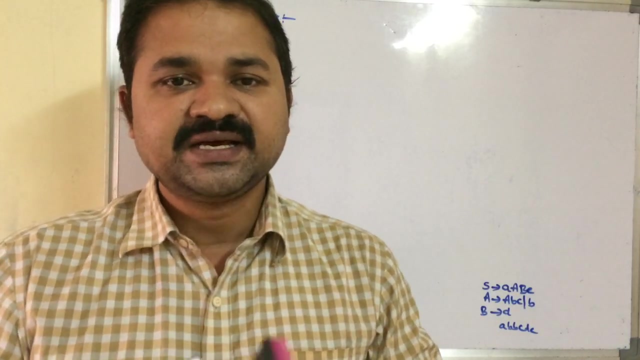 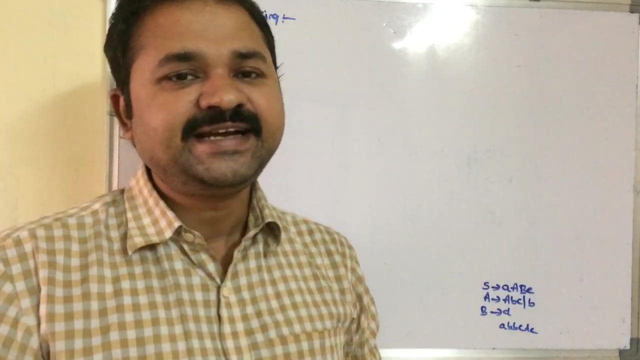 The parser will check whether the token syntax is correct or not. If the token's syntax is correct, then the parser generates parse tree, Suppose. if the token's syntax is not correct, then the parser reports error messages to the user. So the major duty of the parser is it checks whether the token syntax is correct or not. 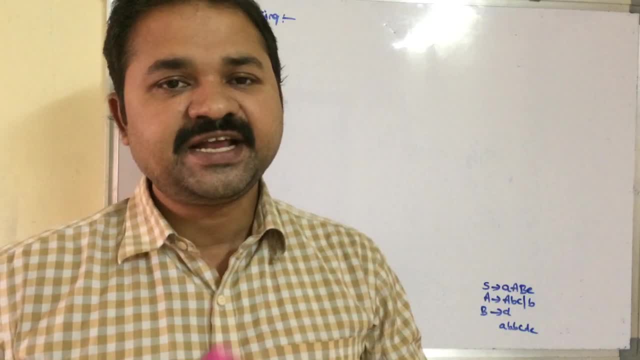 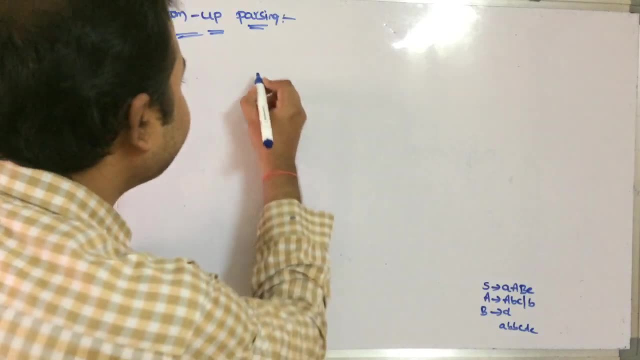 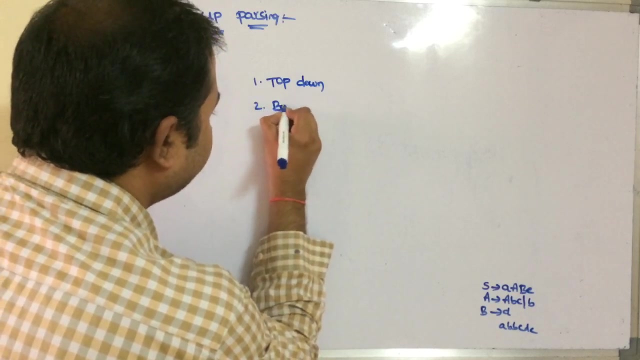 If the token syntax is correct, then it generates parse tree. If the token syntax is not correct, then it generates parse tree. Mainly, there are two types of parsing techniques are available. First technique is top-down parsing technique. Second technique is bottom-up parsing technique. 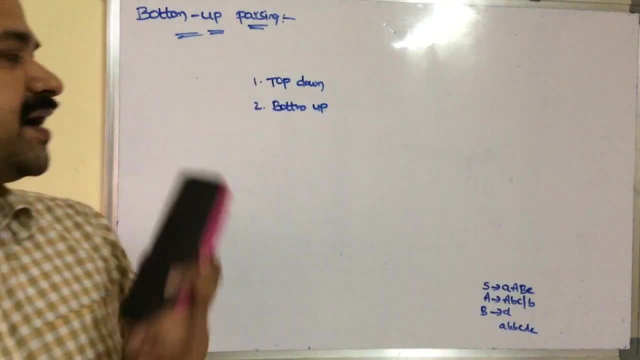 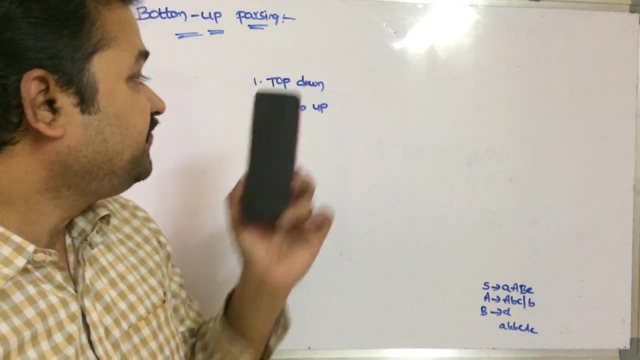 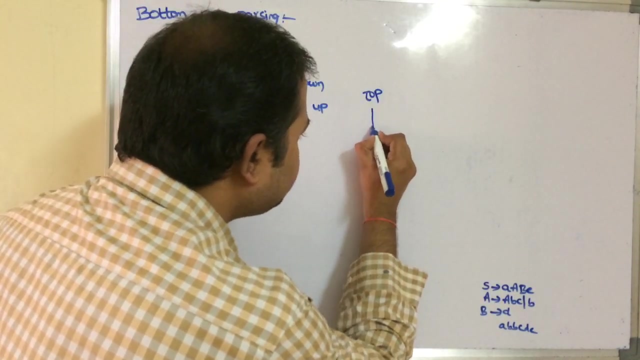 So we have two types of parsing: Top-down parsing and bottom-up parsing. So let's see what is top-down parsing. In top-down parsing, what will happen is the parser will construct the parse tree beginning from top And goes towards down. 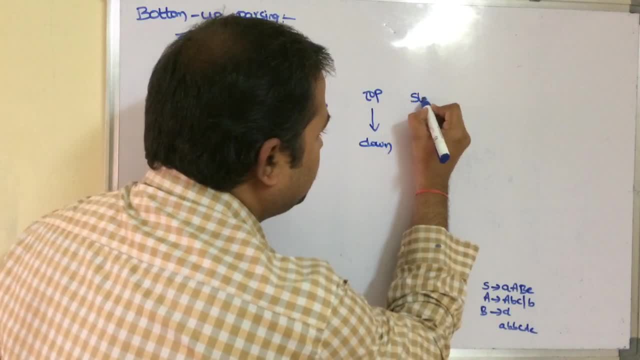 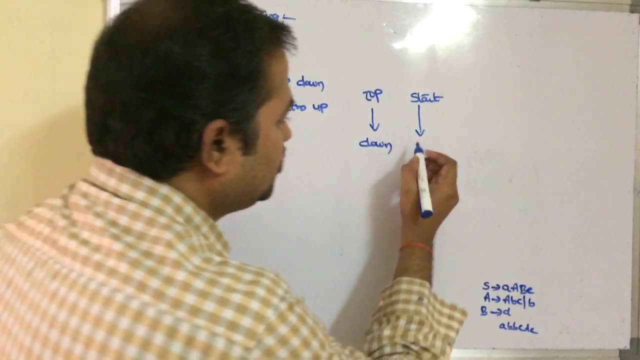 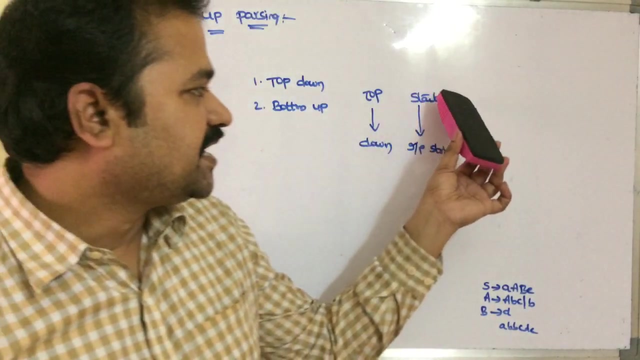 Here top is nothing but start symbol. So the parse tree will be constructed from the start symbol And goes towards the bottom, the down. So the down is nothing but input stream. So for top-down parsing the input is start symbol. 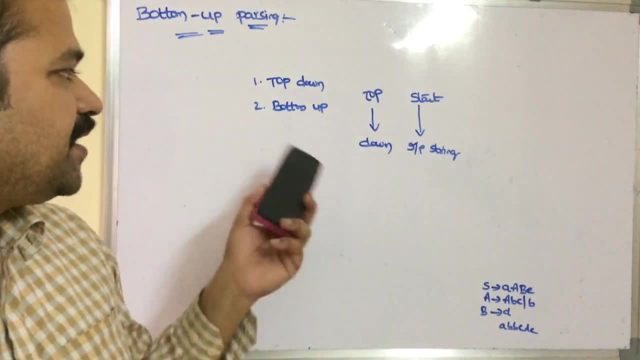 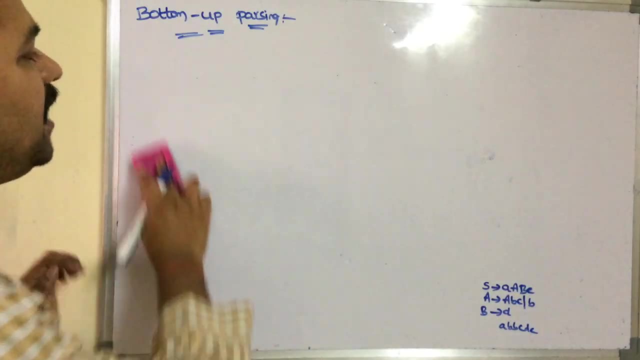 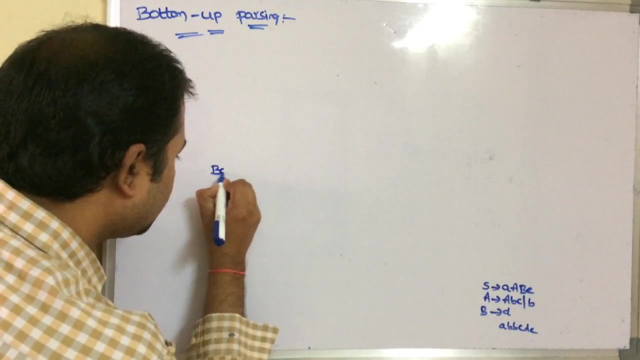 Whereas the output is input stream. Now let's see What is bottom-up parsing. So bottom-up parsing is reverse to the top-down parsing. Bottom-up parser constructs parse tree beginning at bottom. Here bottom means leaves nodes. 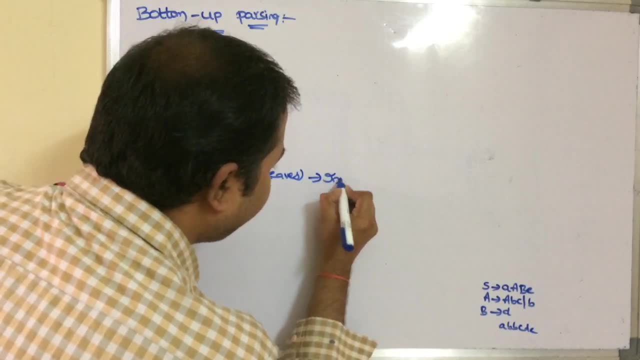 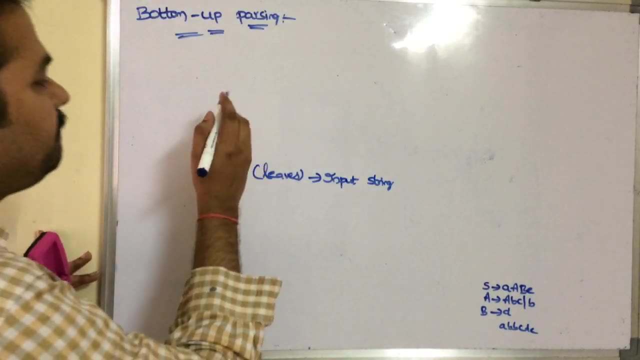 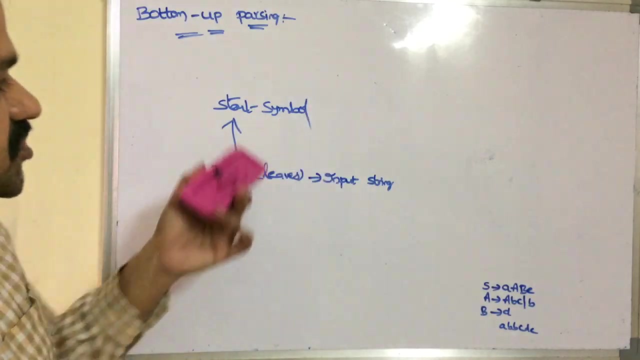 Leaves. So leaves are nothing but input stream And goes towards up. Up means root node. Here root node is nothing but starting symbol of the grammar. So starting symbol means first prediction. left hand side, non-determinant. 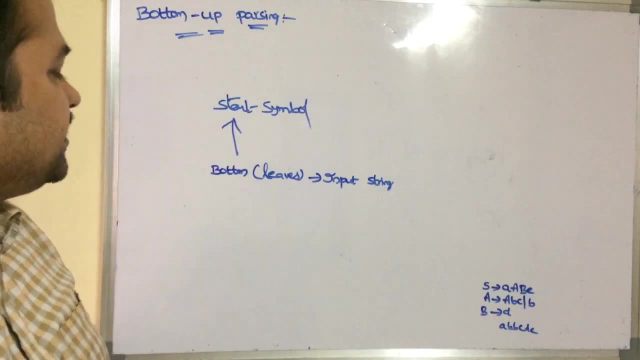 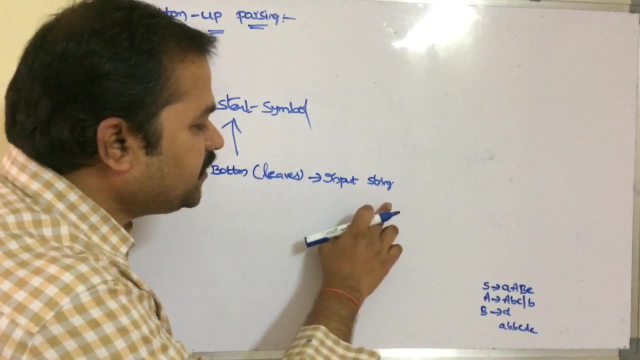 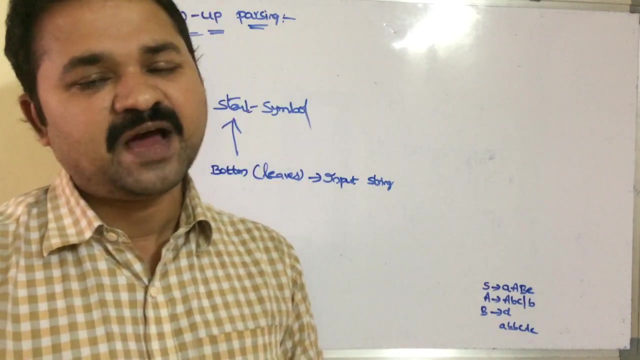 So we can say that bottom-up parser constructs parse tree beginning at bottom leaves that is nothing but input stream And goes towards the root node. Root node is nothing but start symbol of the grammar. So for bottom-up parser, 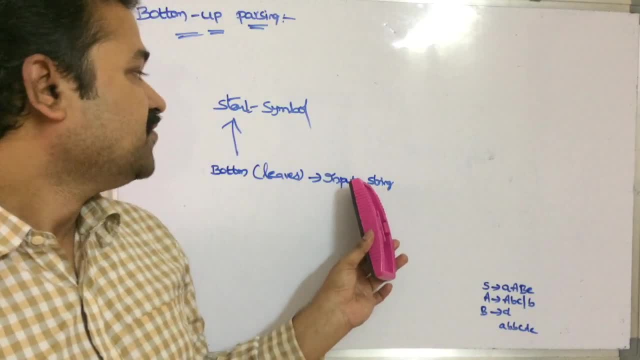 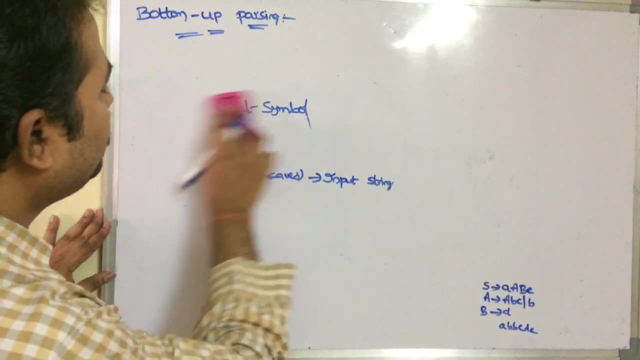 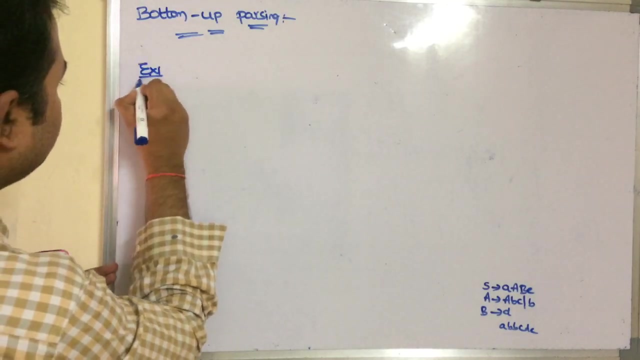 the input is input stream, Whereas the output is start symbol of the grammar. With the help of an example, we will discuss bottom-up parsing in detail. So let us take an example, Example 1.. Let the first prediction is: S implies A, A, B, E. 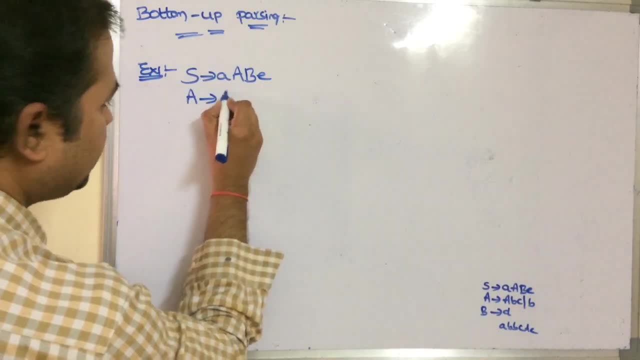 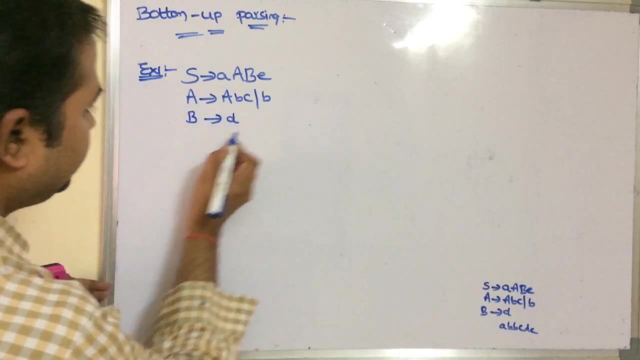 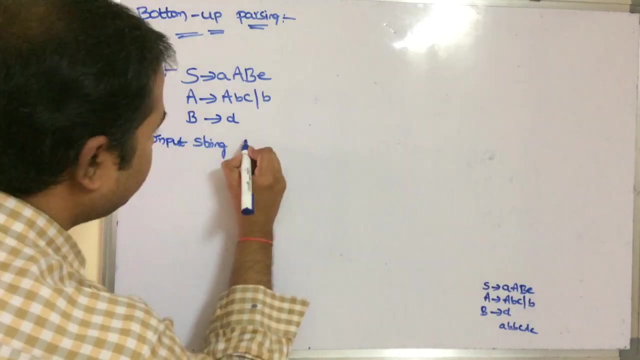 A implies A, B, C. A implies A, B, C. A implies A, B, C. RB, B implies D. Let the input string here is. So we are constructing the parse tree for the input string A, B, B, C, D, E. 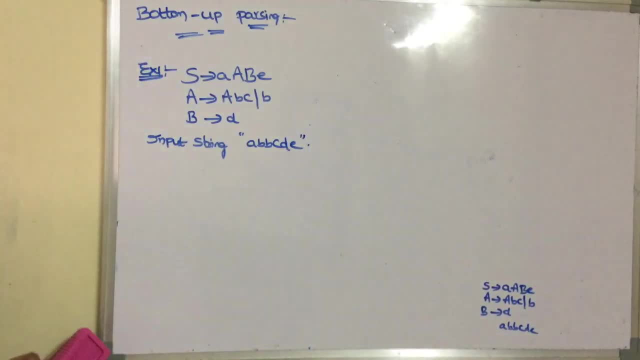 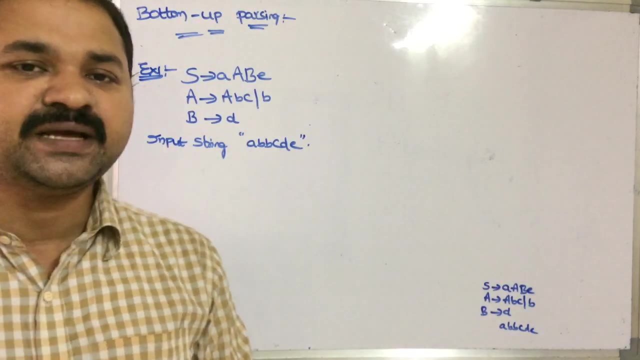 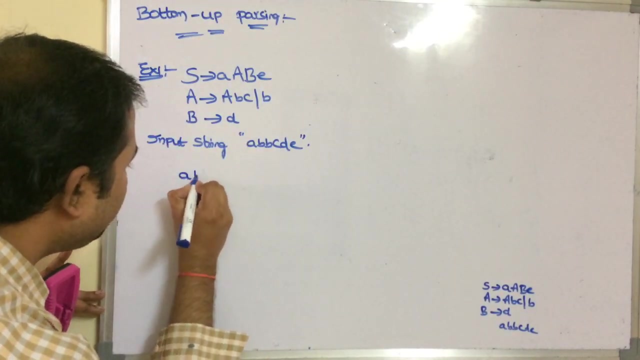 So this is the input string here. Now let us see the bottom-up parsing here. So bottom-up parsing means it constructs the parse tree beginning at the input string. So here, what is the input string string? A, B, B, C, D is the input string. so A, B, B, C, D is the input string in bottom of. 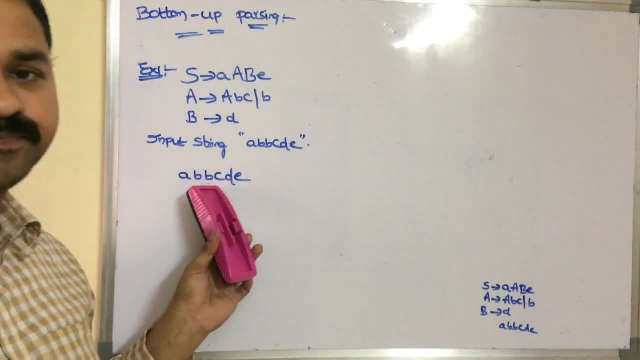 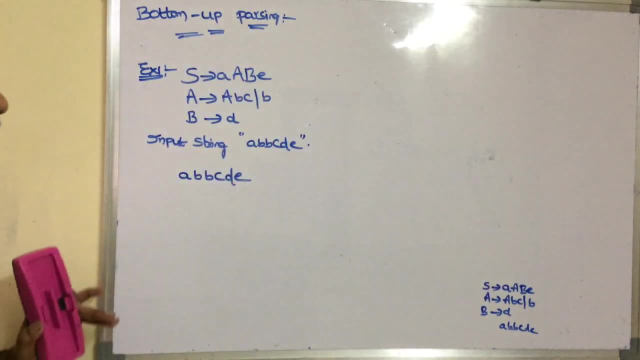 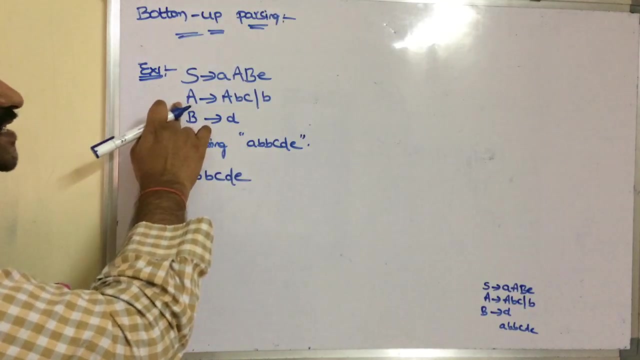 parsing. what will happen is we have to take a sub string and we need to check whether this sub string matches with right side of the production or not. if the sub string matches with right side of the production, then it is replaced with the corresponding left hand side nontripeutal. so initially we have to 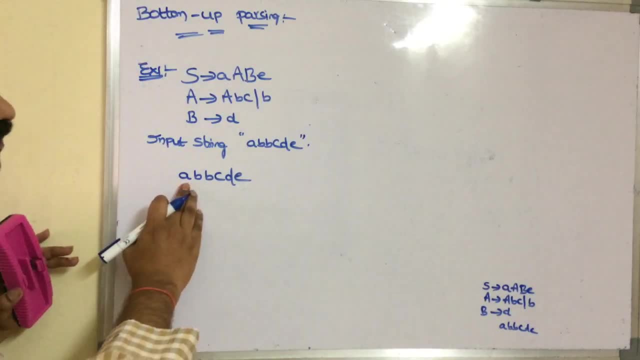 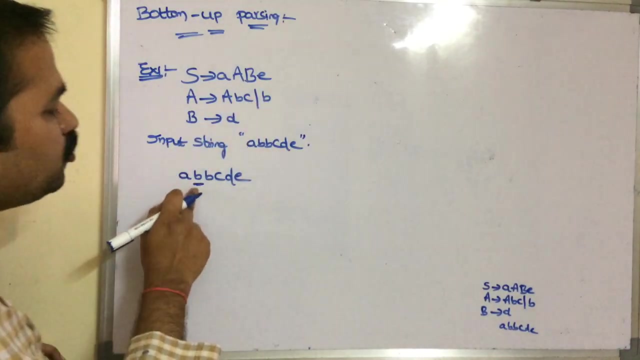 take a sub string. let us take the sub strings as A here. A doesn't matches with right side of any production, okay, no. so now let's take A B, so A- B also doesn't matches with right side of any production. no, let us say B, so B matches with right side of the bluded section. so we have. 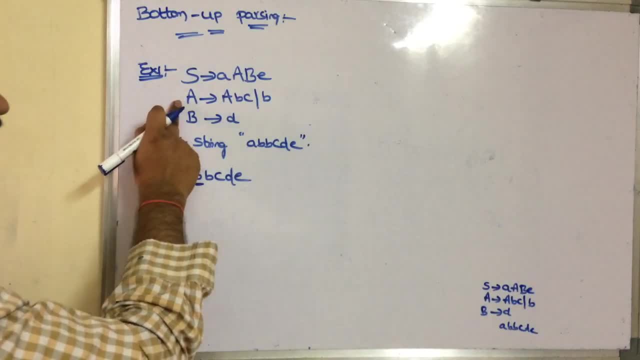 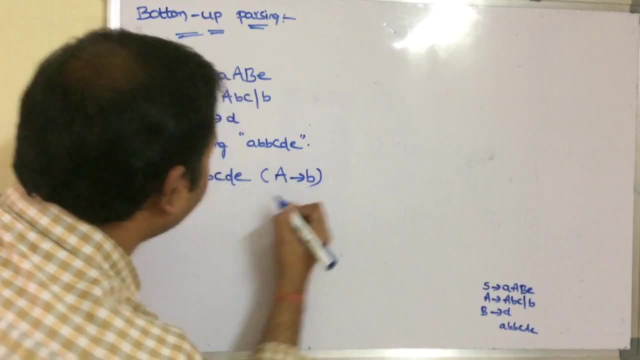 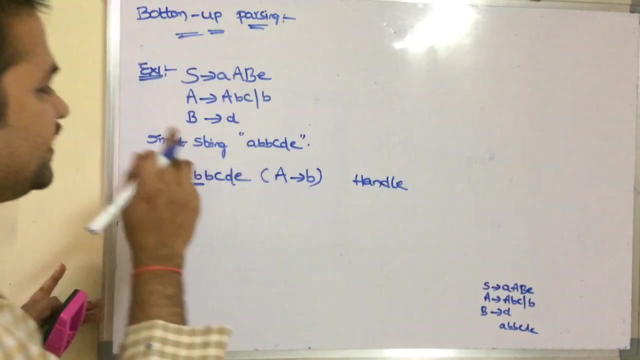 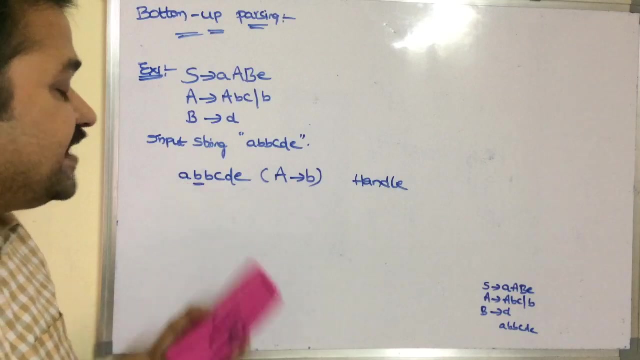 to replace b with the left hand side non-terminal. so what is the left hand side non-terminal? a? so a implies b, a implies b. so here this b is called as handy, so handy is a substring which matches with right side of the projection, and this process is called as reduction. 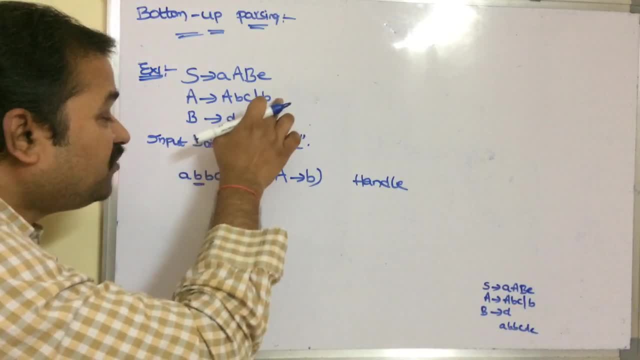 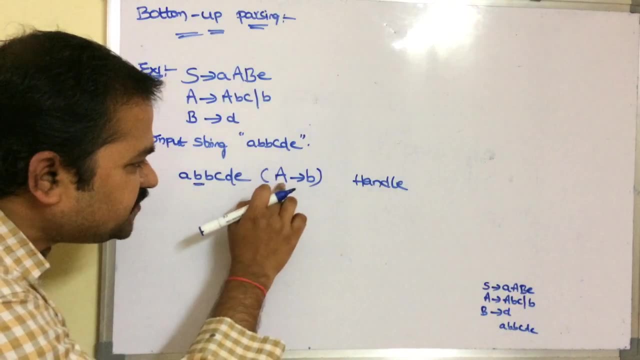 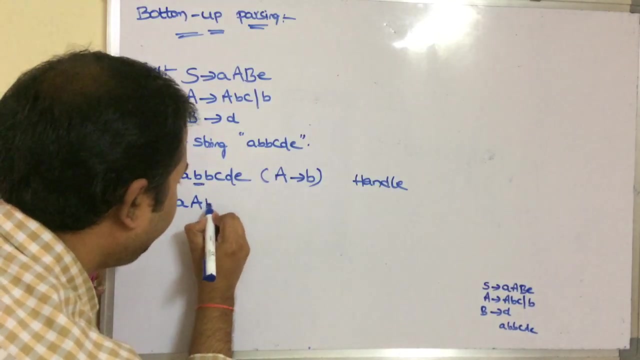 if the subset matches with right side of the production, then it is reduced to the corresponding left hand side. non-terminer here. what is the corresponding left hand side now? terminal capital a. so this b is replaced with capital a. next b, c, d, e. so next we have to take one more. 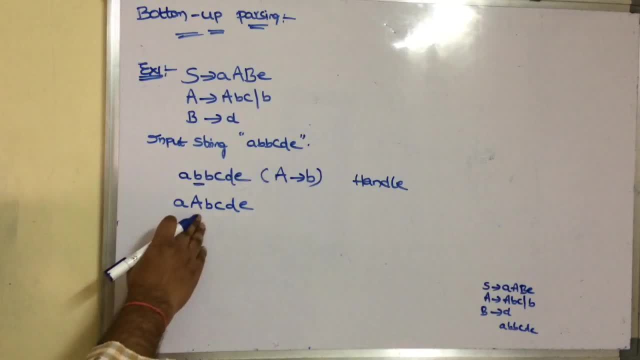 substring. so here, what is the substring we have? uh, here we have b, so b can be replaced with this b, capital, a. so if you replace that one, then what will happen is we will get a, a, a, but a, w is not available here, but here we have abc, so we can take abc as the substring. so we have to replace: 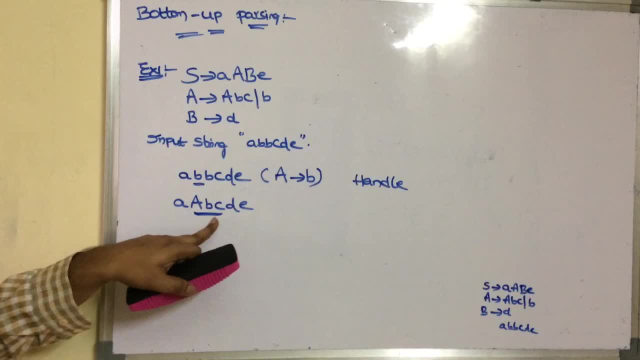 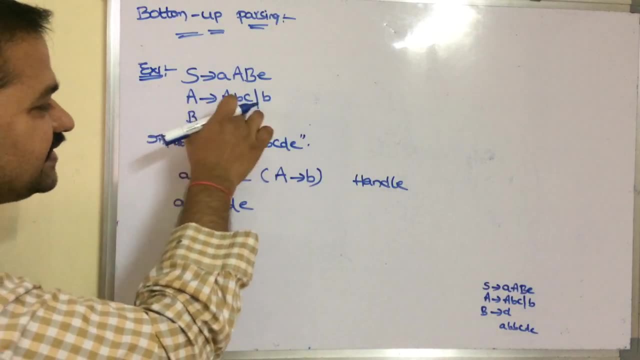 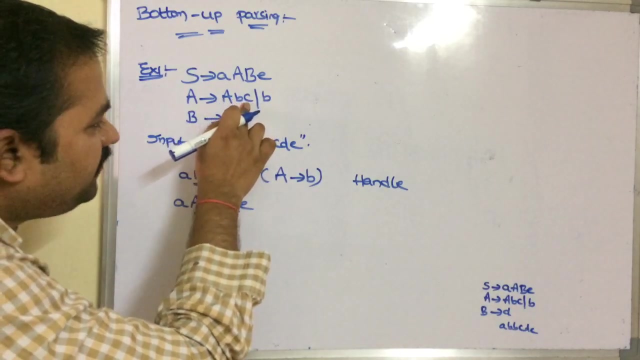 abc with this a. so now we can say that abc is a handle. why? because what is a handle? handle is a substring which matches with right side of the projection. so if the handle matches with right side of the projection, then it is replaced with the corresponding left hand side, not 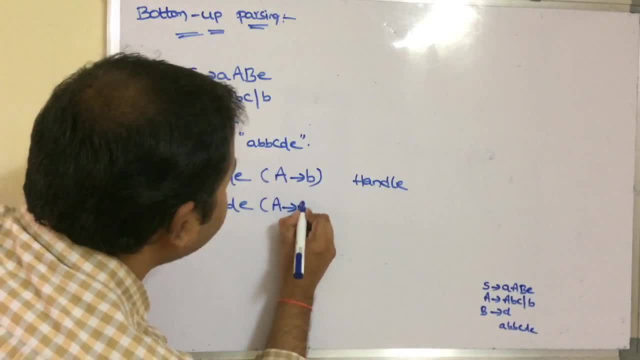 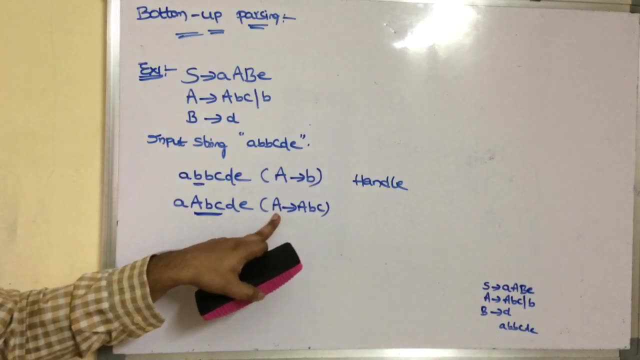 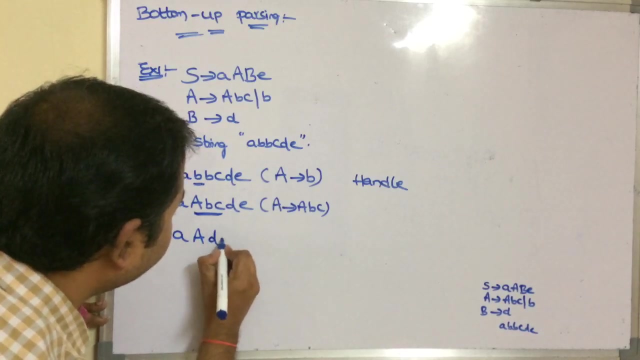 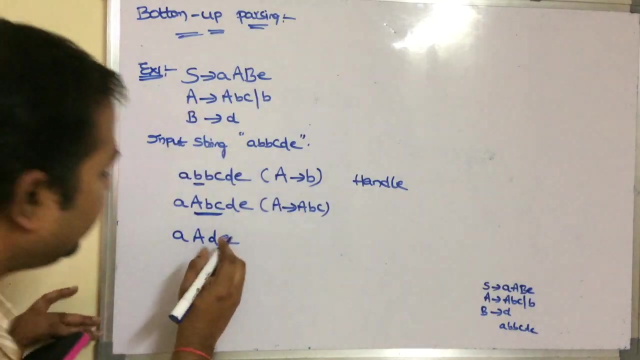 so what is the projection here? a implies abc, is the projection here. so we have to replace this abc with the corresponding left hand side, not terminal. that is a, so a, a, a, a, d, so a, a is not available. a a, d is not available, but here we have d, so this d is available in. 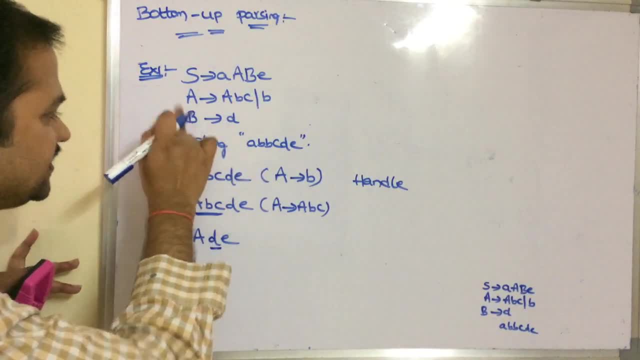 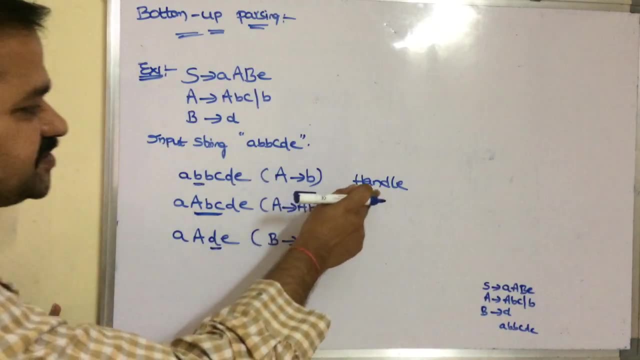 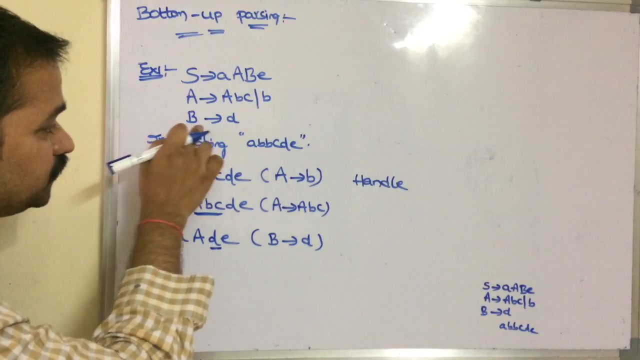 right hand side. so this d is reduced to this b, so b implies d. so now this d is a substring. this substring is called as handy, so whenever the substring matches with right side of the projection, then it is reduced to the corresponding left hand side, not terminal. 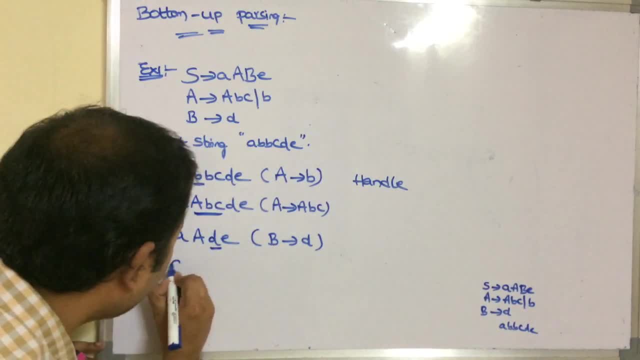 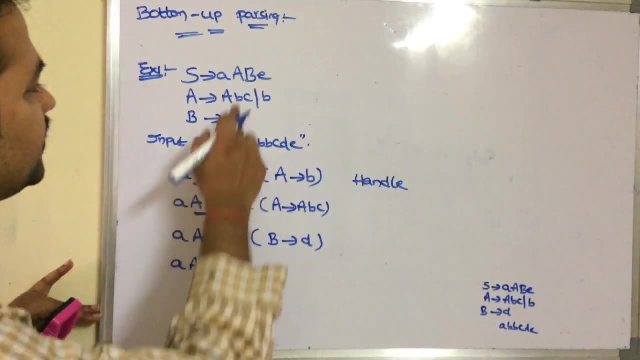 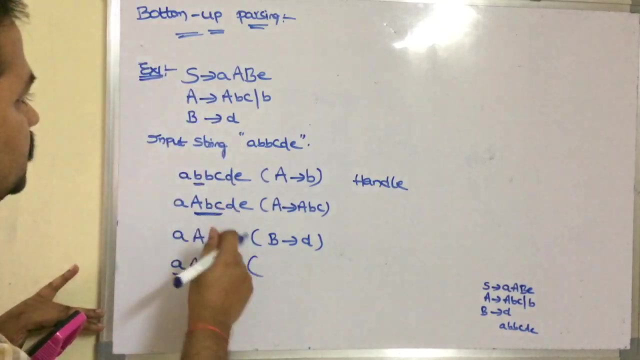 so what is the corresponding left hand side? not terminal b. so a a. so this d is replaced with capital b, so capital b e. so what is a a b e? a a b is nothing but the starting symbol. yes, so now this a, a b e will become the handle. so a a b e is replaced with the corresponding left. 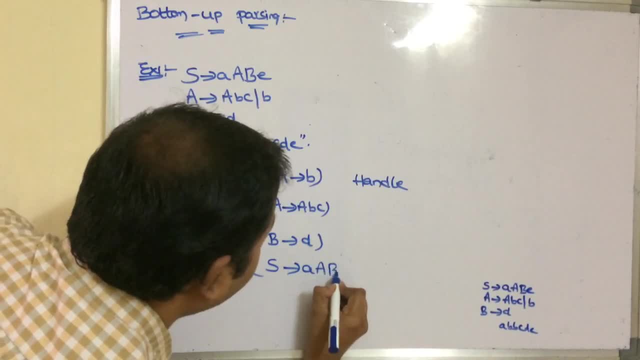 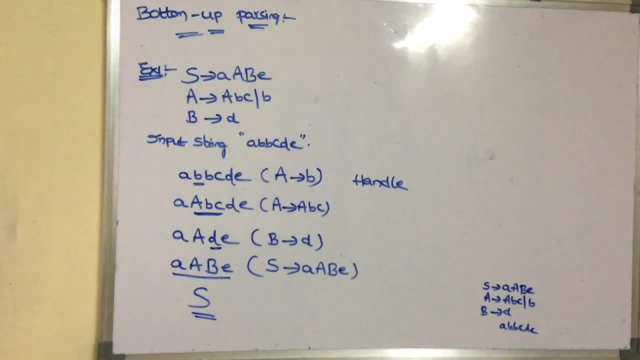 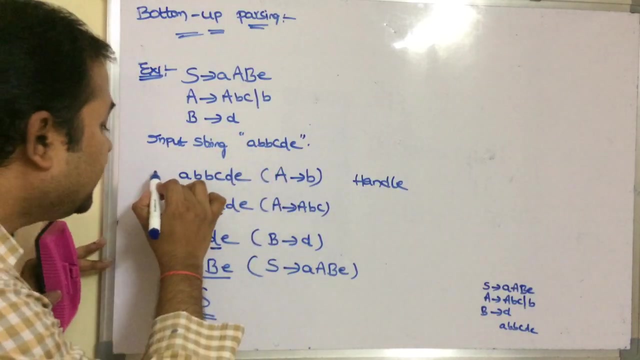 hand side: non-terminal. so yes implies a, a, b e. so a a, b e is reduced to yes. so this is nothing but the corresponding start symbol of the grammar. so in this way we can generate a bottom of passing. okay, so here we can say that bottom of passing is the process of reducing. 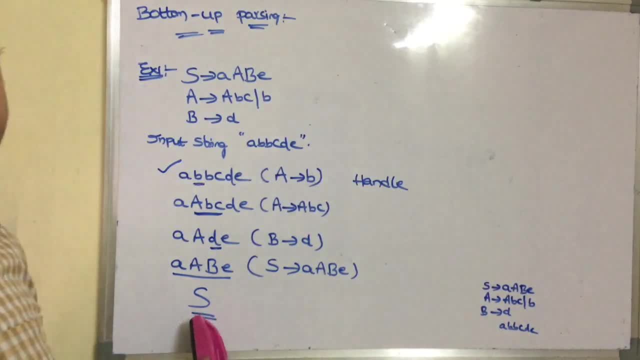 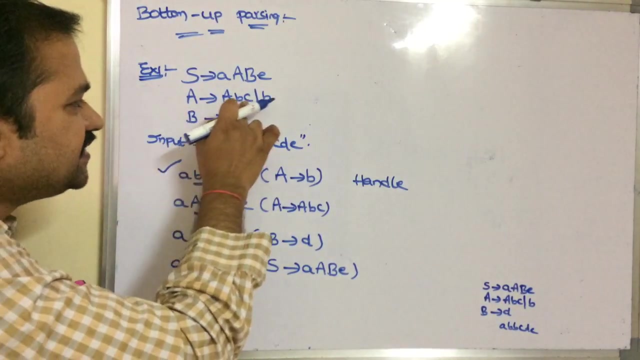 input string to the starting symbol of the grammar. so here we are reducing the input string abb, cde to the start symbol of the grammar. so what is reducing? reduction means if the substring or handy matches with right side of the projection, then it is reduced to the corresponding left hand side non-terminally. 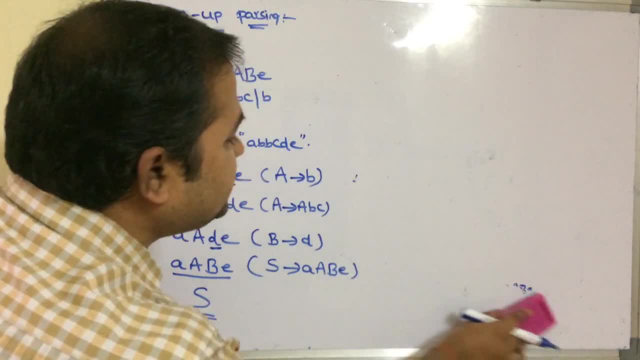 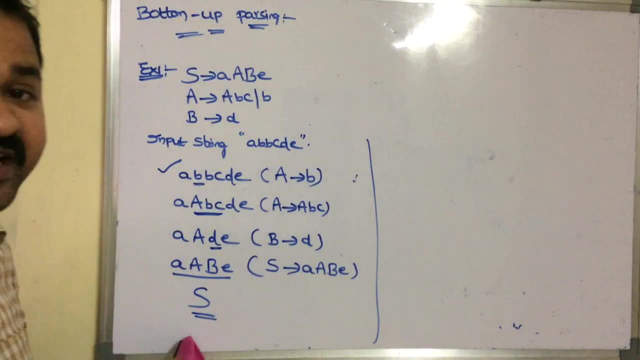 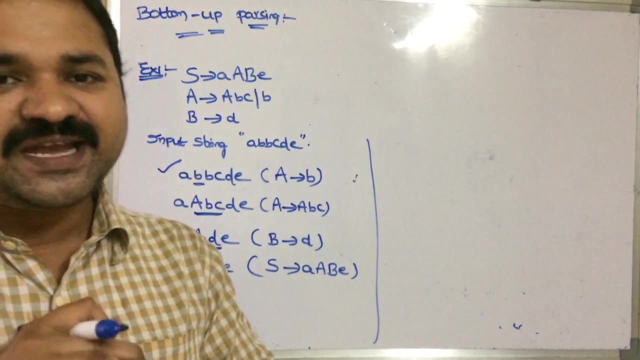 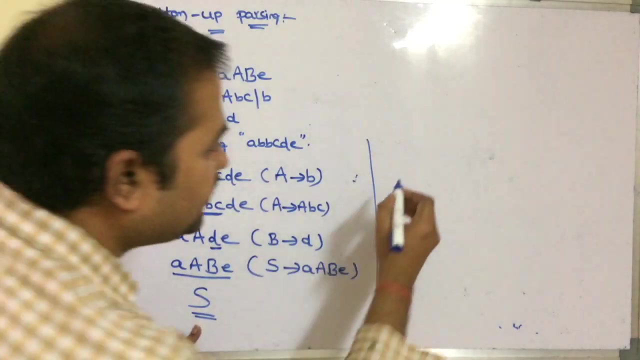 if we observe this derivation, so this derivation is nothing but rightmost derivation in reverse order. rightmost derivation in reverse order. so we have two types of derivations are available: leftmost derivation, rightmost derivation. so rightmost derivation means in each step the rightmost non-terminal is expanded. so here, what is the last step? yes, next s implies. 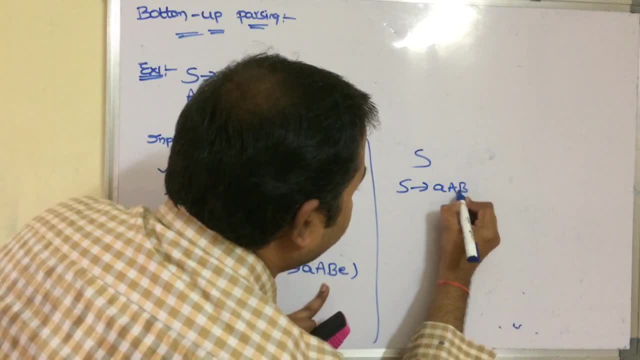 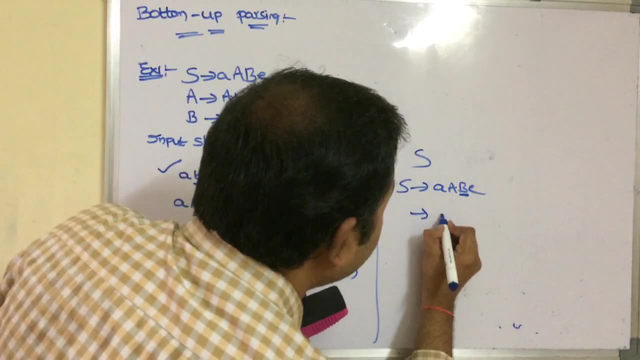 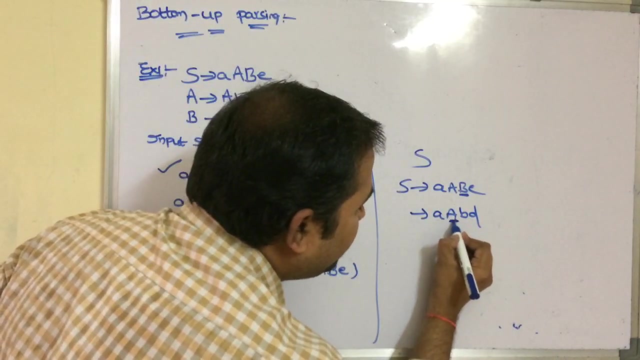 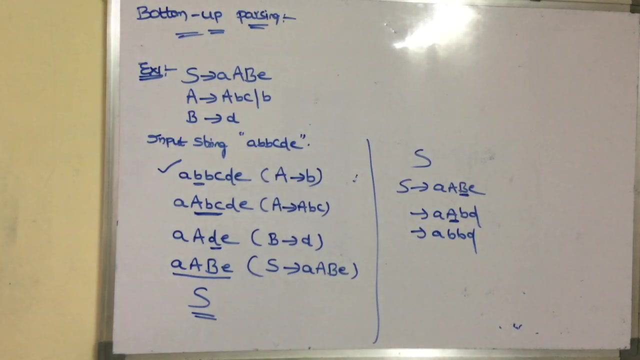 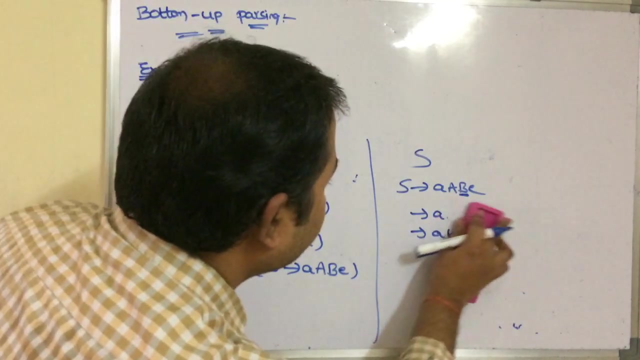 a, a, b e. so s implies a, a, b, e. so what is the rightmost non-terminal here? b is the rightmost non-terminal, so b means d. so a, a, b, d. next, what is the rightmost non-terminal? we have only one non-terminal, that is a. so what is a, b? so? a implies a double b, d, a double b. so here, what is b, a, a, so 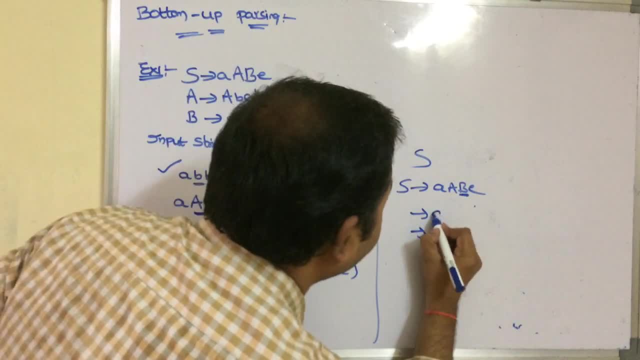 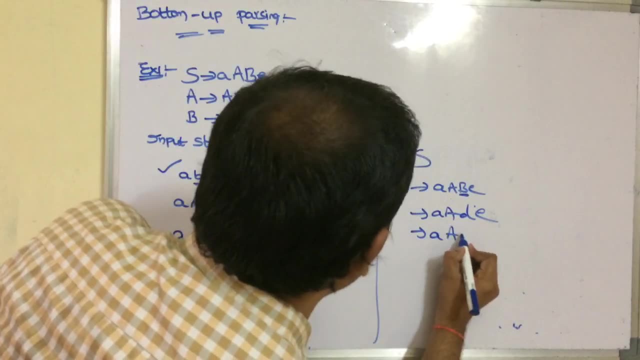 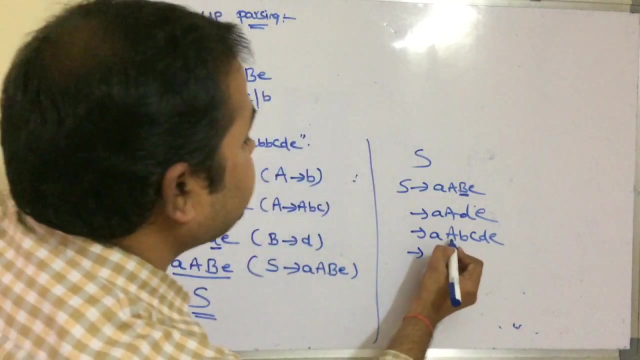 s implies a, a, b, e, so a, a. so what is b? so b means d e. next, what is a, a means a, b, c, d e. okay, next, so what is this a, this, a is nothing but a, b, b, c, d e. so this is nothing but our input string. 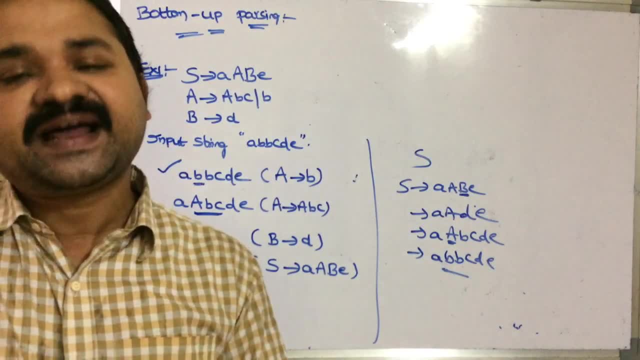 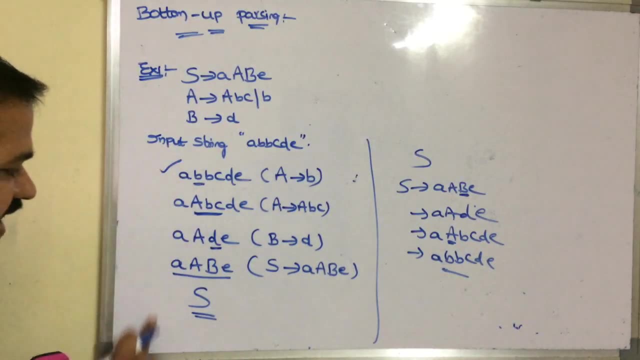 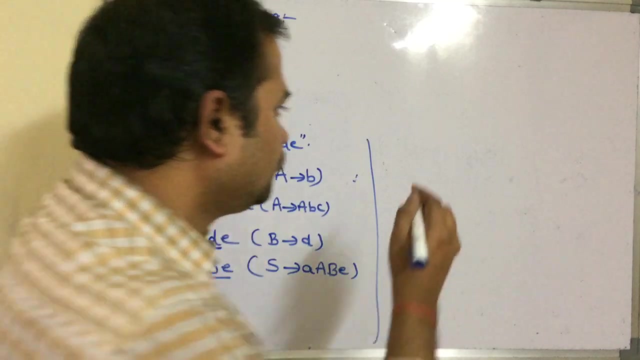 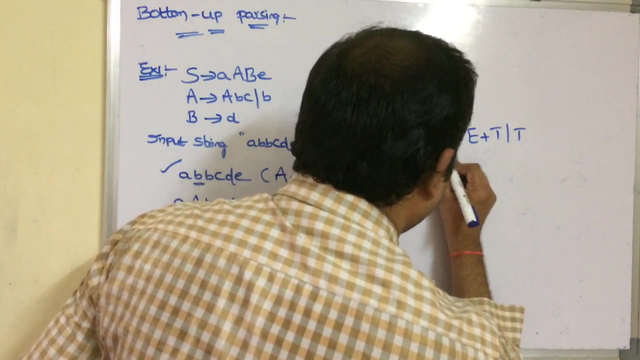 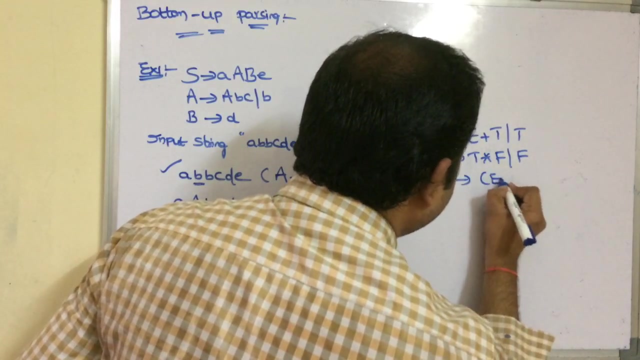 so we can say that if we select the substring correctly, then the bottom of parser will generates the rightmost derivation. so this is nothing but the rightmost derivation. in which order? in reverse order. so let us take one. now let us take another example. e implies t by t, t implies t star, f by f. f implies left parenthesis, c, right parenthesis by id. 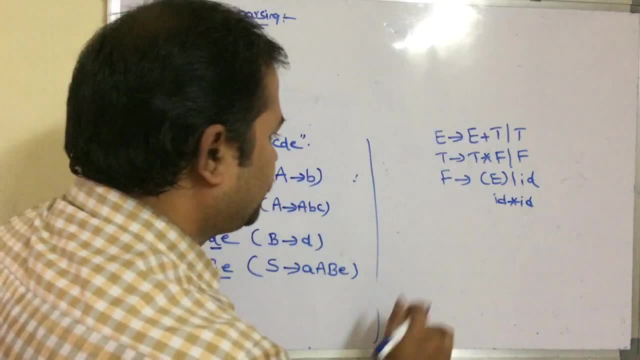 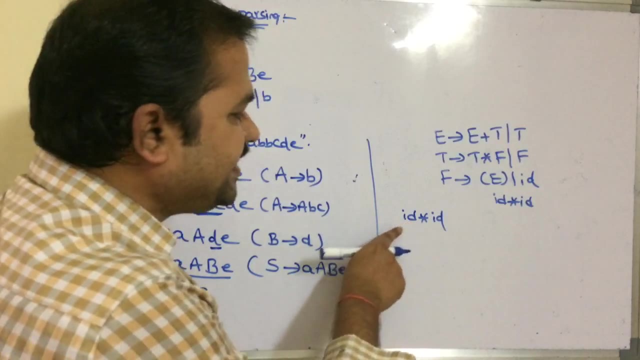 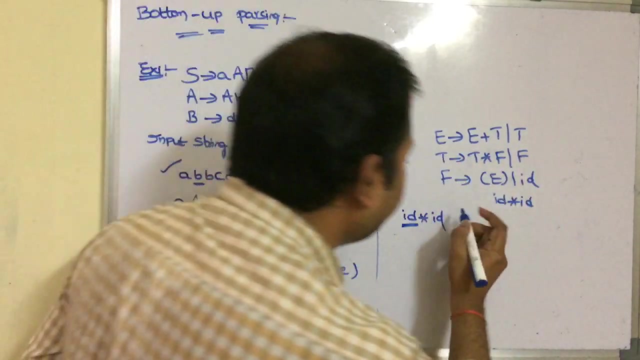 so let the input string is id, star id. so let the input string is id, star id. so first we have to take a substring. let the substring is id. so id is available in right side of the projection. so what is the corresponding left hand side? non-terminal f. 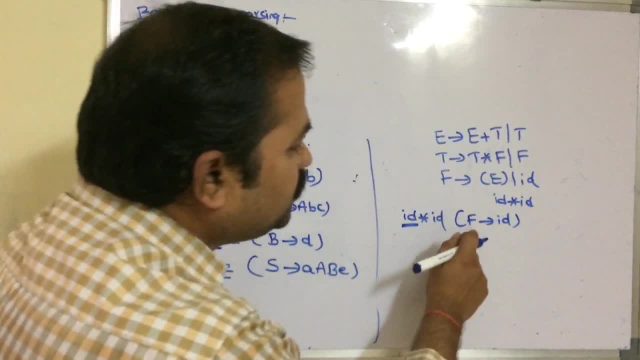 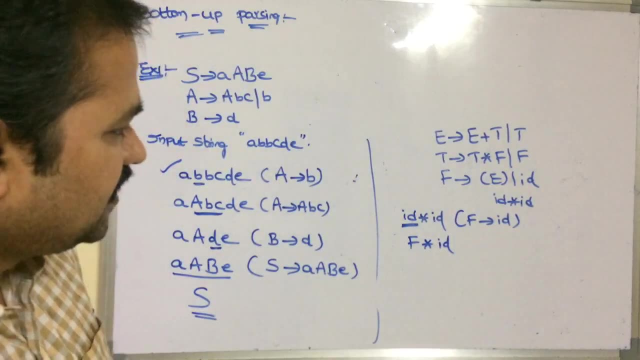 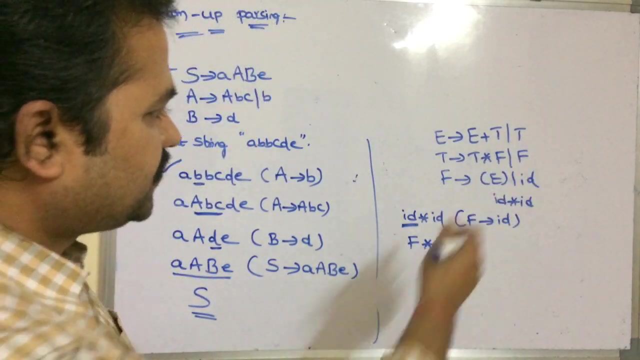 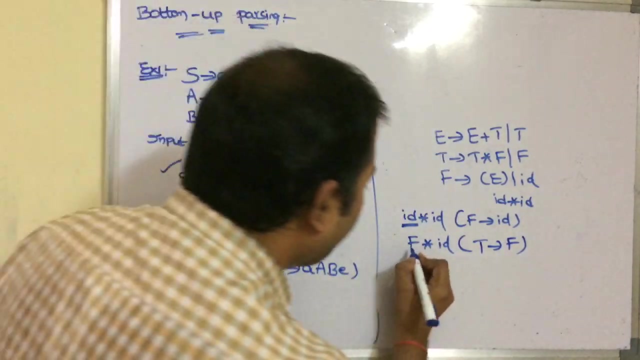 so f implies id. so this id is reduced to f now, so f star id. next we have f and f star id. so here f is available on right side of the production, so we can reduce f to t. so what is the corresponding production for f, t? so now, reduce f to t, so t star id. 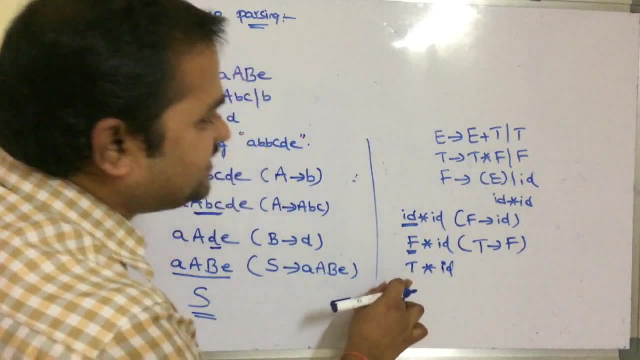 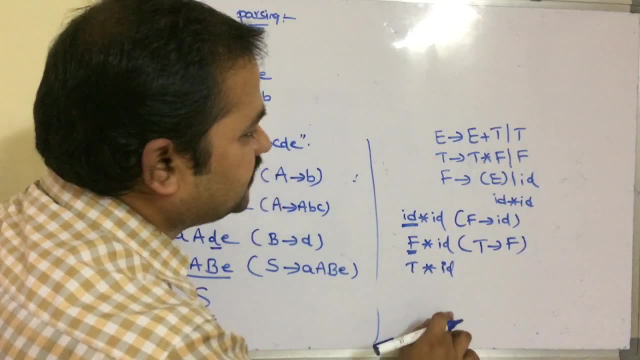 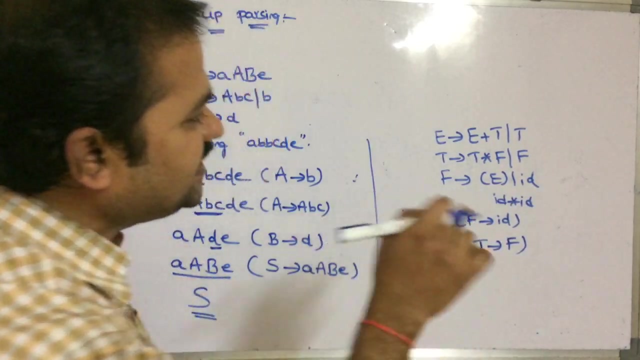 t star i. so next, if we take t as the substring, then what will happen is t is reduced to e, then we will get e star id, e star id. so e is not available here, but id is available here. so id is replaced with f, e star f, but we don't have e star f in the right side of the production. 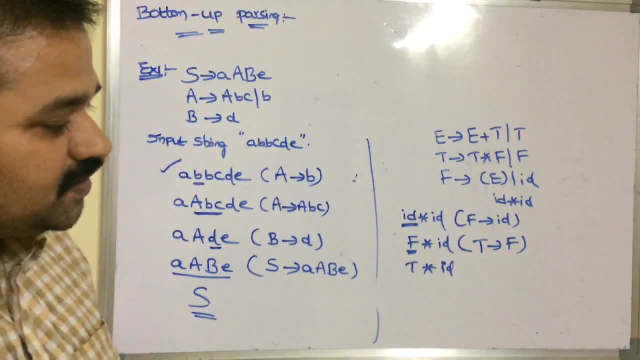 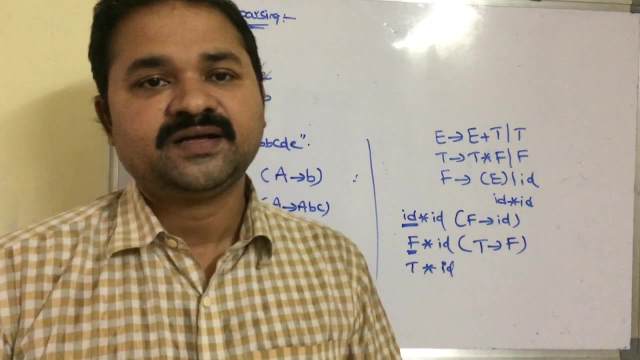 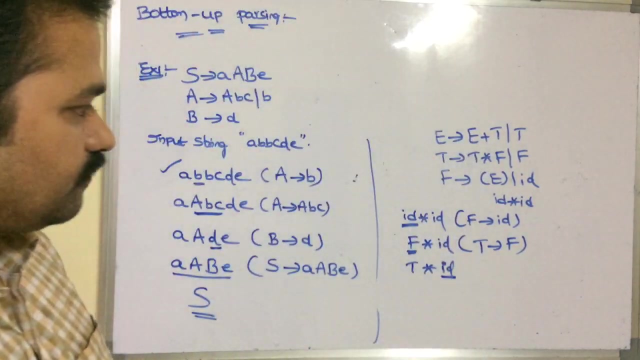 so we should not consider t as the substring here. so here, while generating the bottom of parser, we have to consider the correct substring. then only we will get the star symbol of the grammar. so here the correct substring is id. so for id, what is the corresponding left hand side? non-terminal f implies i. 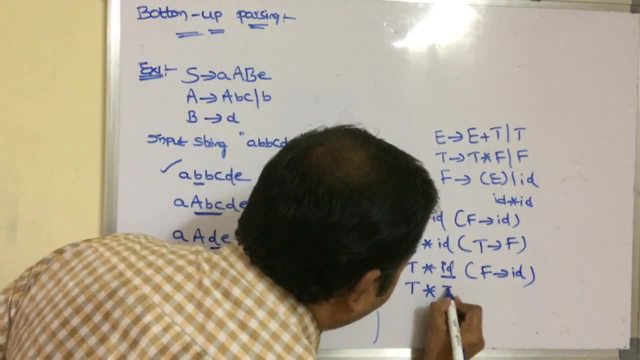 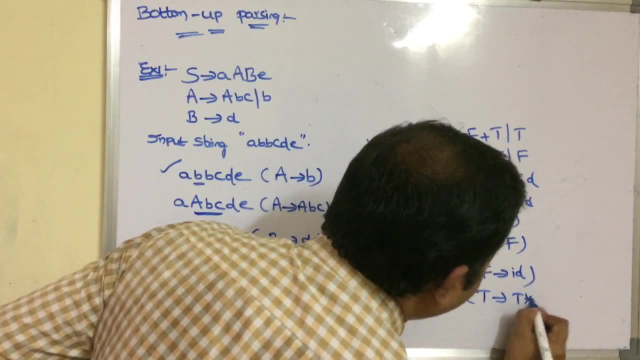 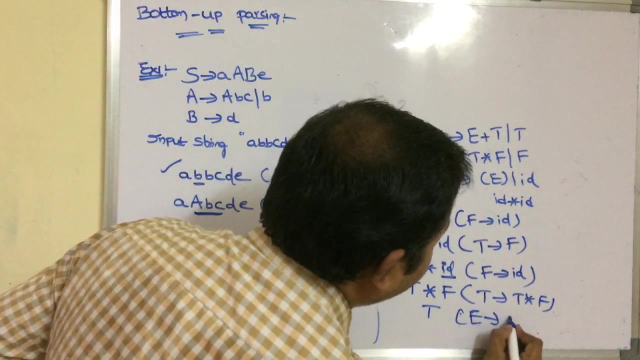 so id is reduced to f, so t star f. so what is t star f? t star f is nothing but t, so t implies t star f. so now t star f is reduced to t. next, what is t? so t is nothing but e, so t is reduced to e. 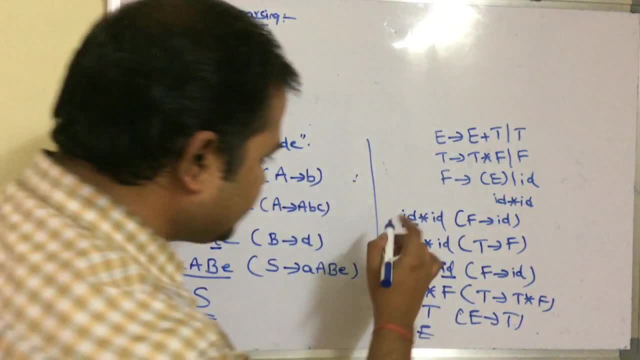 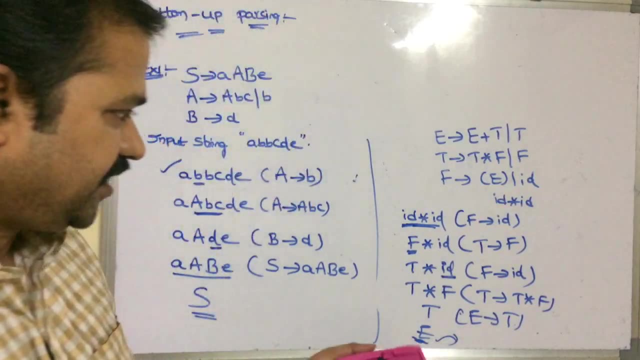 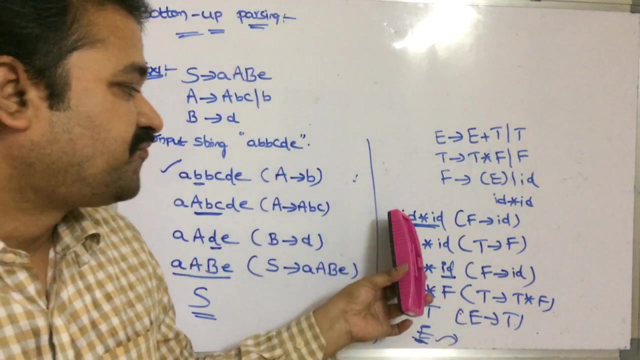 so in this way we can generate the bottom of passing. so here, what is the input here? id, star id is the input string, whereas what is the output here? e is nothing but the output. okay, so here we have three important points. so bottom of parser constructs the parse tree for an input string. 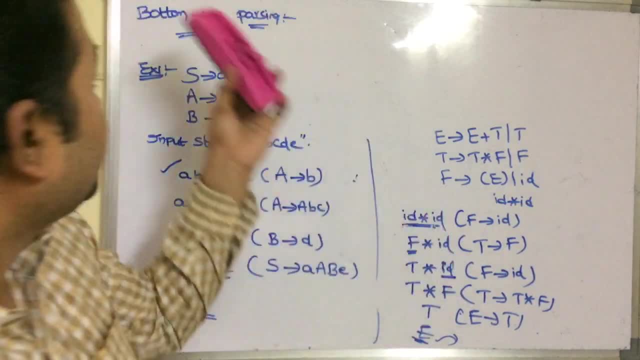 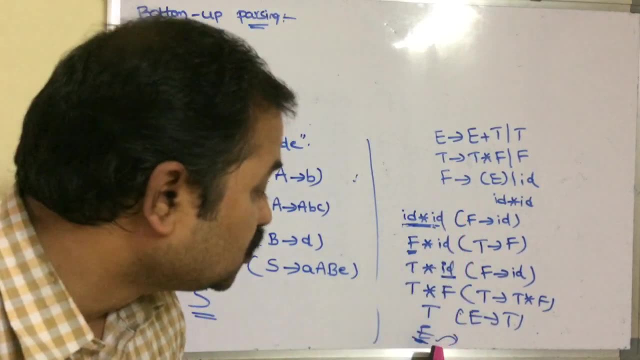 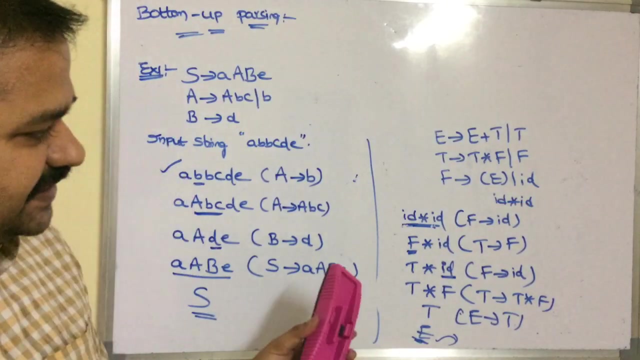 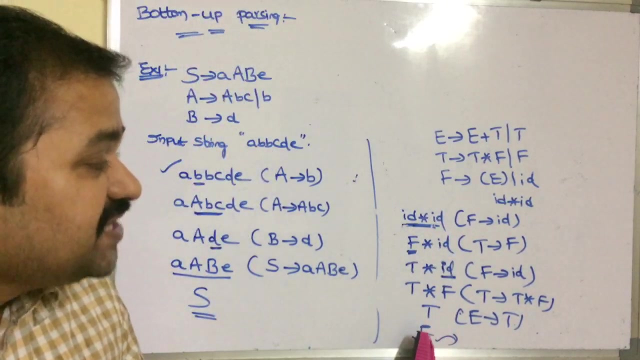 beginning, yet beginning, yet the bottom. so the bottom is nothing but leave notes, that is nothing but inputs and goes towards to the root. so root is nothing but start. symbol of the grammar. and we can also say that bottom of parser is the process of reducing input string to the start symbol of. 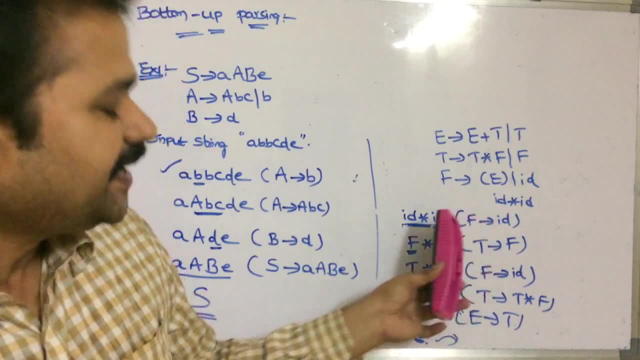 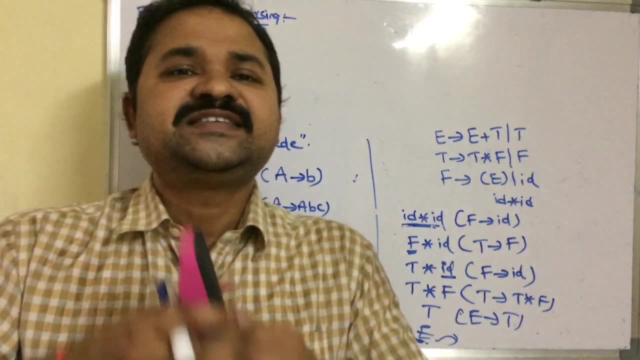 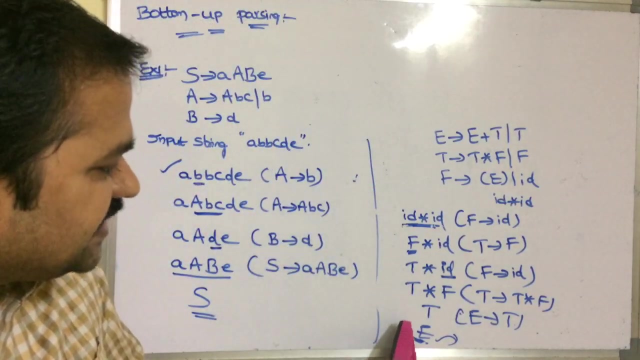 the grammar. so id, star id, is the substring, input string, whereas e is nothing but start symbol of the grammar. and one more point here is: if we select the substring correctly, then bottom of parser produces the rightmost derivation. so this is nothing but the rightmost derivation in reverse. 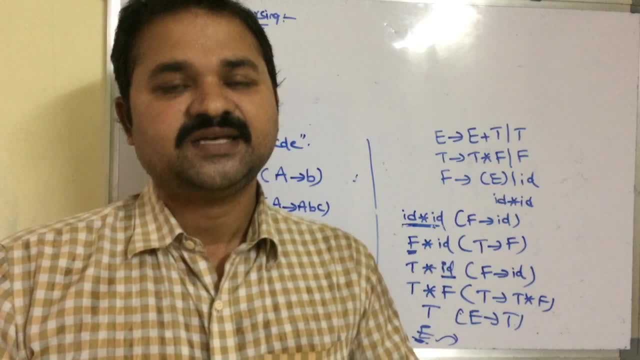 order, the rightmost derivation in reverse order. so this is about what is bottom of.